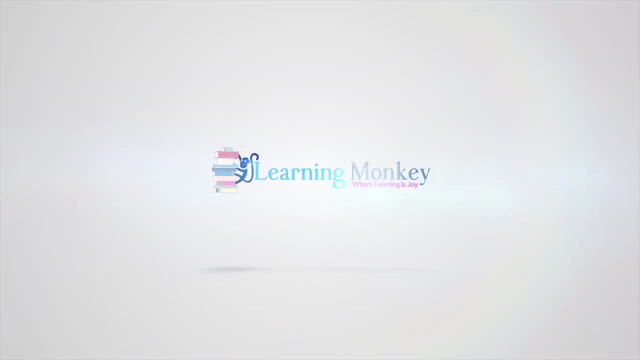 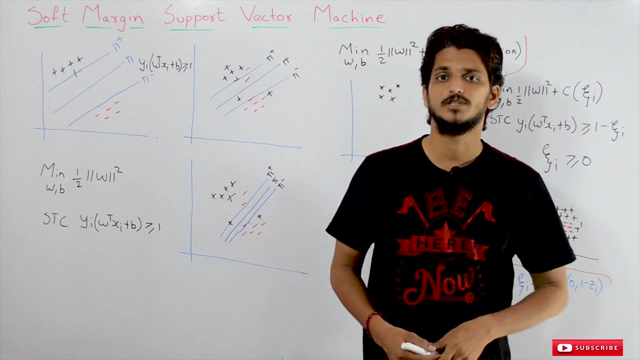 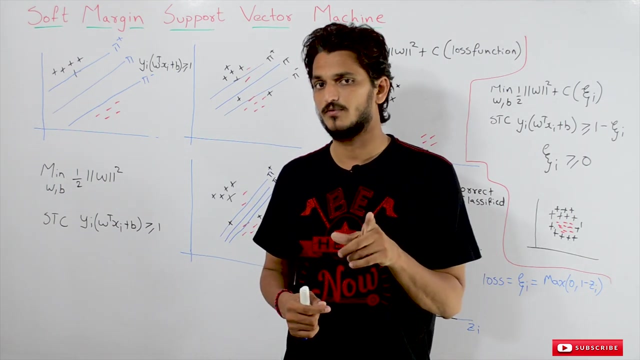 Hi, welcome to Learning Monkey. I am Raghuvir. In this class we will discuss about soft margin support vector machine. In our previous classes we already discussed about hard margin SVM and we defined the optimization problem for hard margin SVM and we defined the solution. 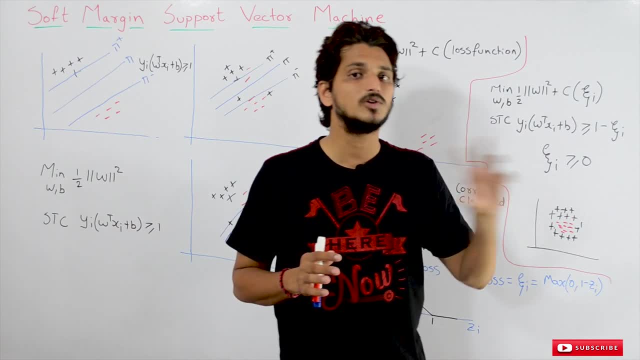 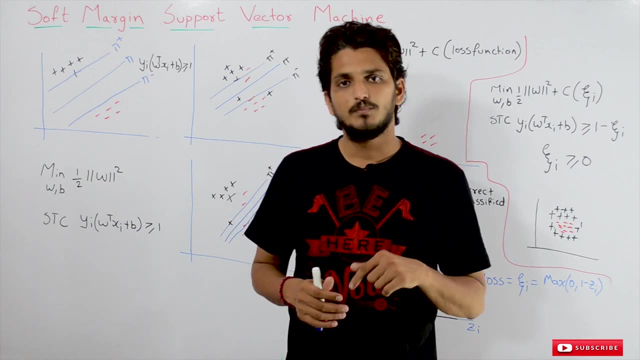 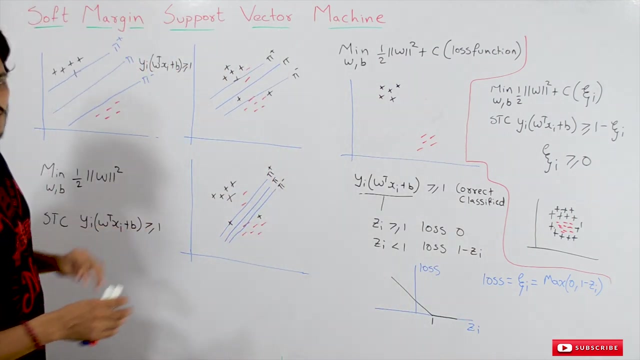 how to solve this optimization problem also. So please watch our previous classes and come back here. Those concepts are very important for understanding this class, So the link for the playlist is provided in the description below. Before going into the concept of soft margin- SVM, let's refresh the concepts of hard margin SVM for a minute. Then we go into. 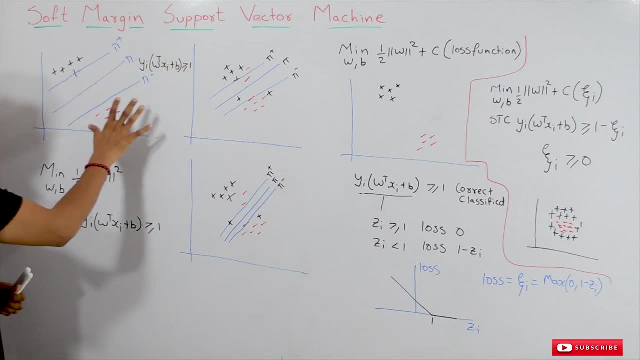 the concept of soft margin SVM. The assumption which we considered in hard margin SVM is the data set is linearly separable. So what's the goal of SVM is it will identify a line. Suppose this is the line which is identified by our support vector machine, It will identify. 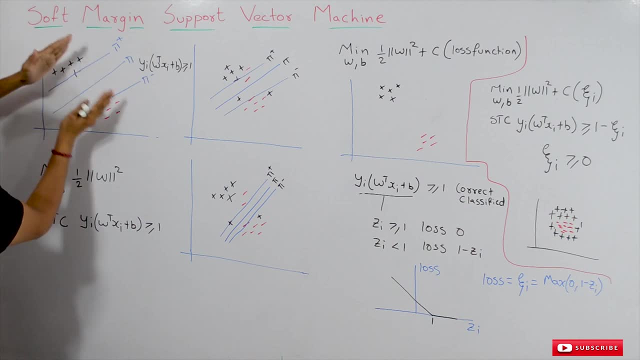 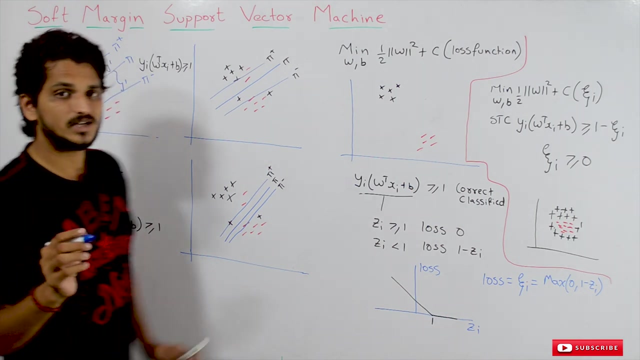 a line that maximizes this geometric margin. This geometric margin, that's the line identified by support vector machine. So it will identify a line that maximizes this geometric margin, But the functional margin is one. Don't Don't get confused with functional margin and geometric margin. Our goal of support: 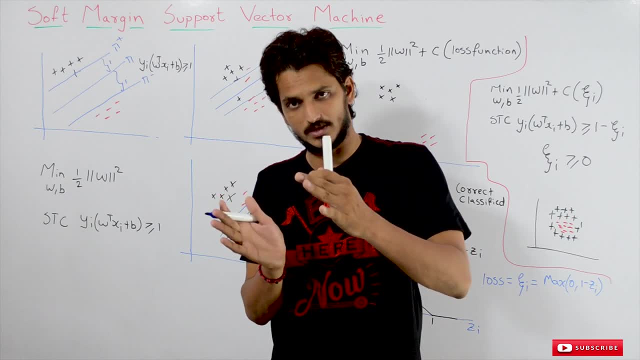 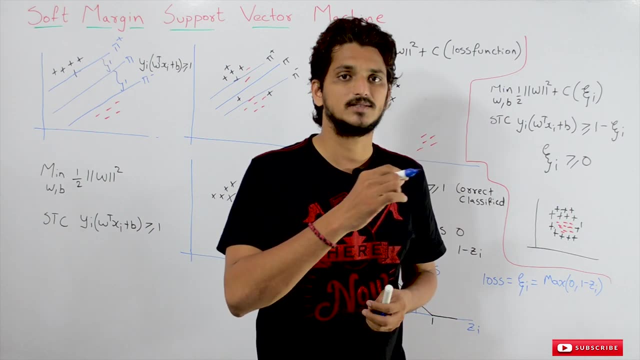 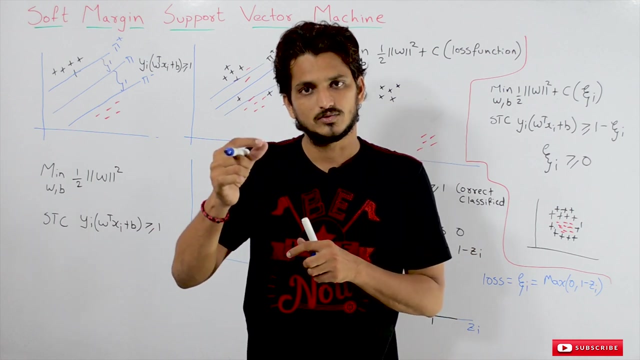 vector machine is to identify a line that maximizes the geometric margin. But the functional margin will be one, because that's what we clearly discussed in our previous classes. We will adjust the functional margin. We can adjust any way and we'll make it as one. So 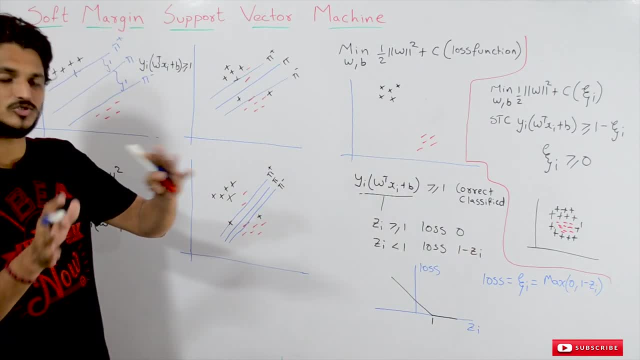 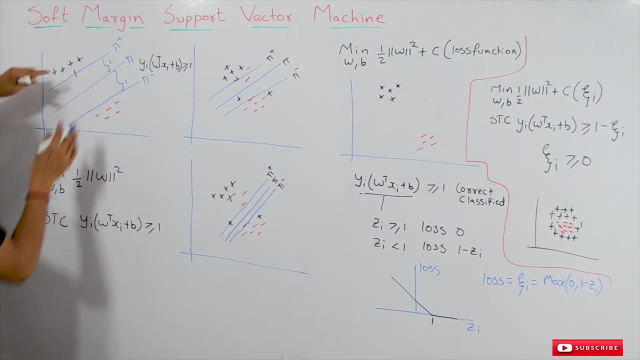 functional margin is one, But geometric margin. we cannot change the geometric margin, It is constant for any thing. Okay, Yes, So functional margin is one, So we'll identify a line that maximizes this geometric margin. So the optimization for problem for this is given as the minimum of W, B means we will. 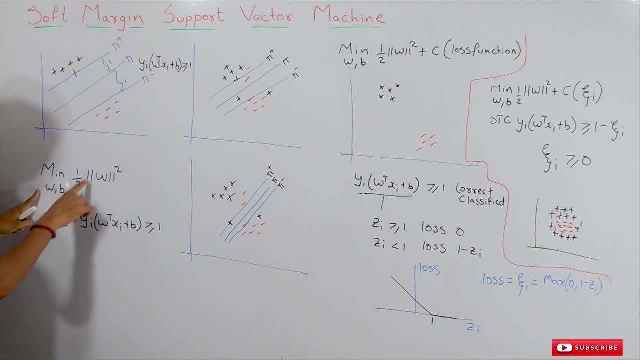 identify a line that minimizes this one by two into no more W square. If if you are trying to minimize, this means we are trying to maximize the margin subject to constraints. Yi W transpose Xxi plus B greater than are equal to one. So these are the constraints y To the bicycle. 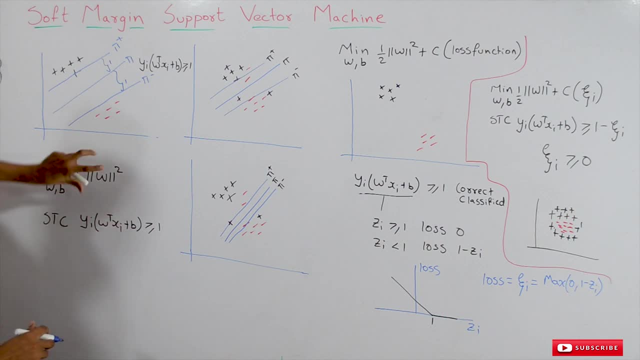 that will A first be good. then, like people, we have a afin Thought is I have to answer. so these are the constraints we have and we are trying to minimize this. this is the optimization problem which we discussed in our hard margin svm. and one more important point: we have to 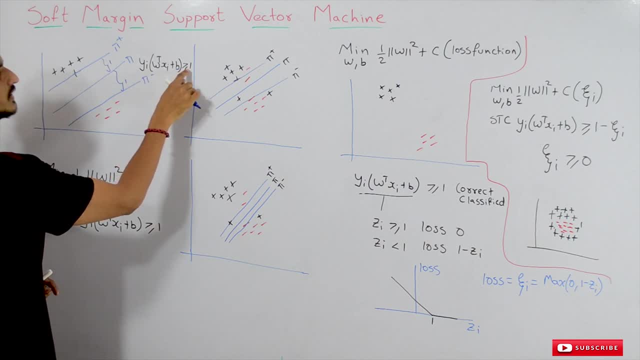 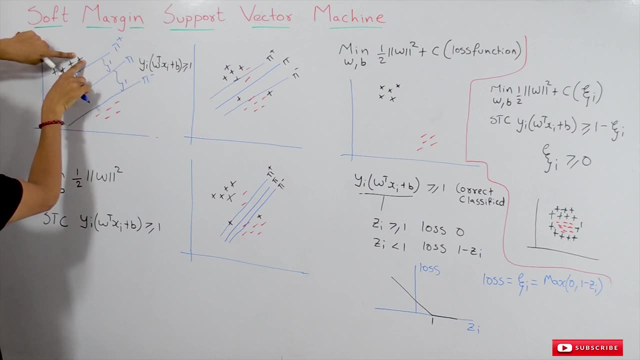 understand. here is yi w, transpose xi plus b greater than or equal to 1? what's that mean? suppose, take this point: what's the actual value for this yi value positive means plus 1 into, if you substitute this point in this equation, what's this equation, this line equation? 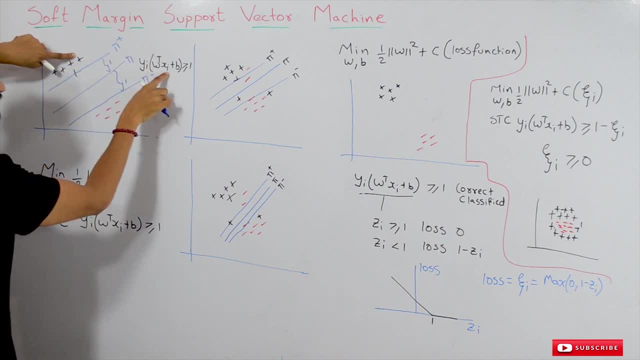 if you substitute this point values in this equation, what we are calculating? we are calculating the functional margin. the functional margin because this point is on this side. the functional margin value will be positive. positive into positive. positive if it is greater than or equal to 1 means if our point is above this line. above this line means correctly classified. 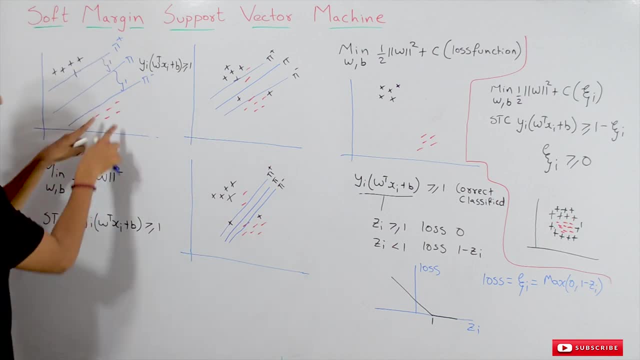 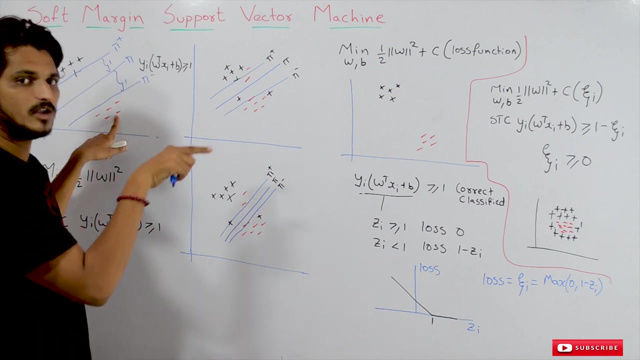 correctly classified. the same way, if you take a point, this side, negative point, means yi value is minus 1. if you substitute this in this equation, we will get a functional margin value of negative value, negative, into negative positive, and if that value is greater than or equal to 1 means correctly classified. correctly classified: this concept is very 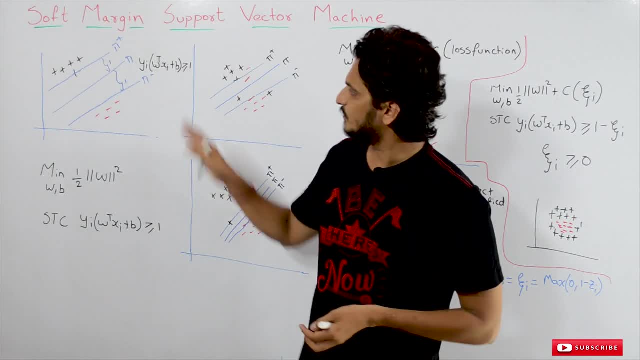 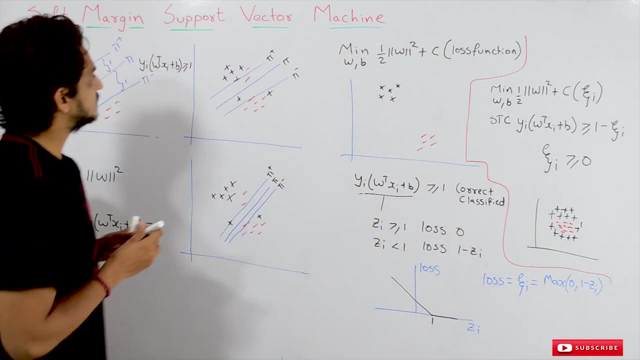 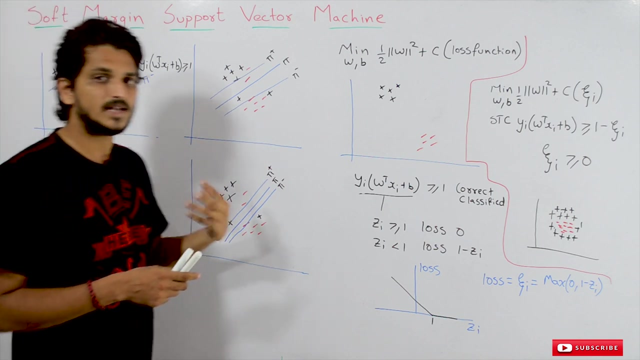 helpful in understanding a soft margin svm. that's why we repeated this concept. we discussed this concept in our previous classes svm also. so, coming to soft margin svm, before going into the optimization problem, first have a graphical intuition so that you'll have a better understanding of optimization problem. so what soft margin svm means, we will. 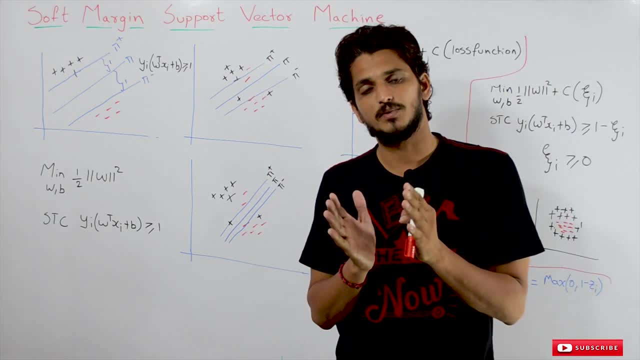 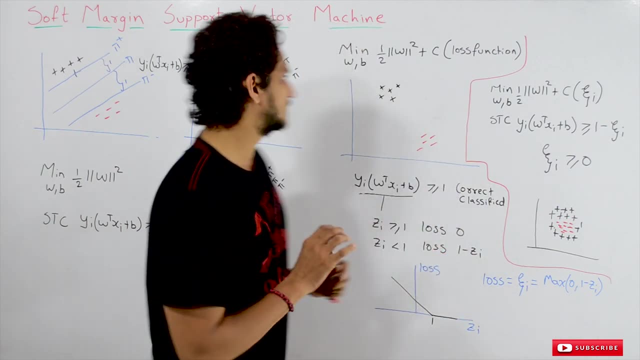 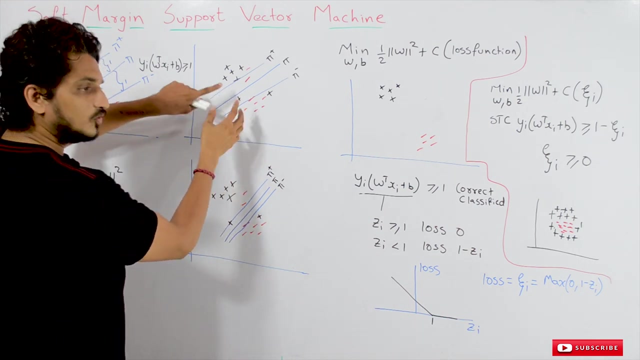 take out that exemption, our data set is linearly separable. we don't take that exemption means our data set is not linearly separable. so let's take an example: data set, this data set. if you consider this data set, these two are same data sets. you you take, you identify any. 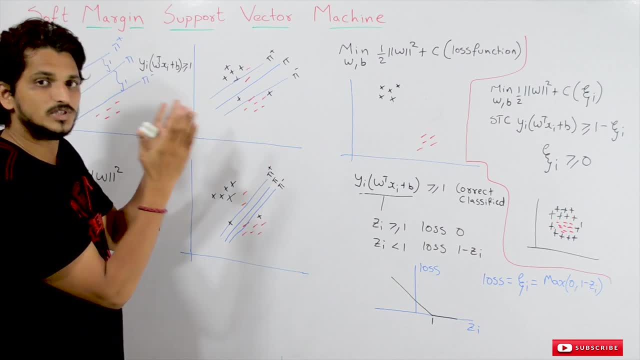 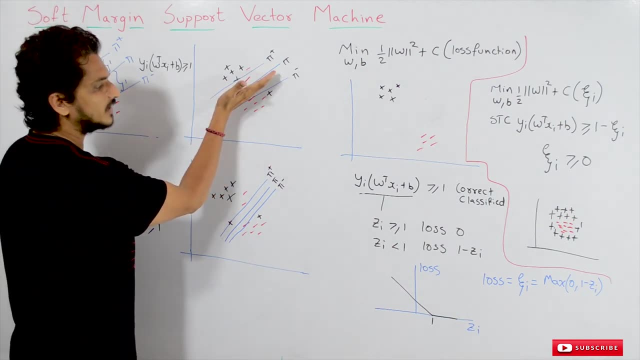 line, but we cannot separate positive and negative points using that line. that is what not a linearly separable data set means. a first suppose: if I identified this line as the best line, I say that this is the best line, but someone, some other person, will say that this is the. 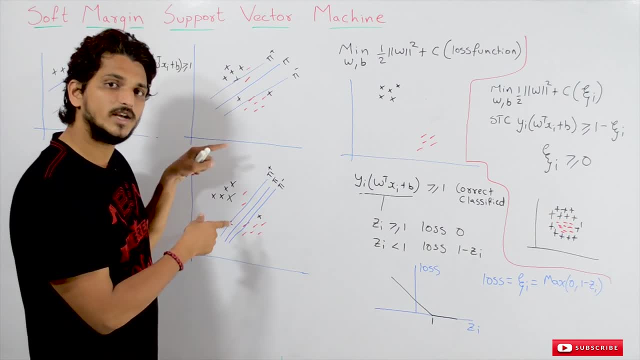 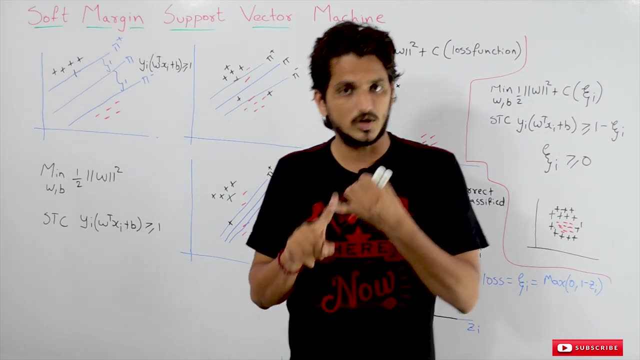 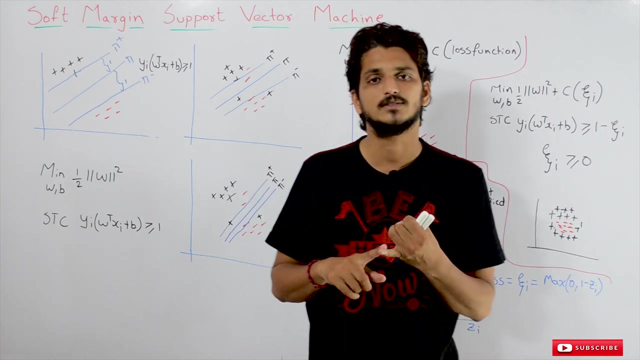 best line. how can we say that? which one, which one we have to identify? the same question arises in our previous problems also, when we discussed about a logistic regression. we can identify multiple lines. which line we have to identify? what we have done in our previous classes? in logistic regression we defined a loss function. 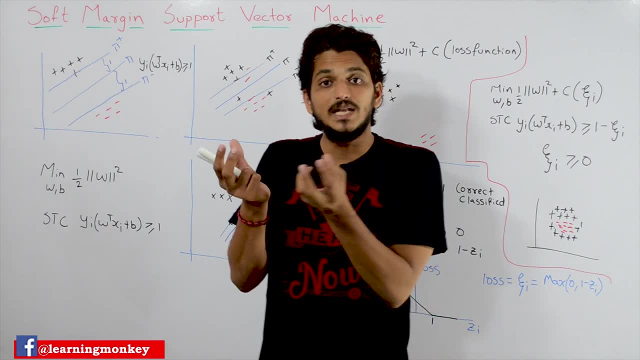 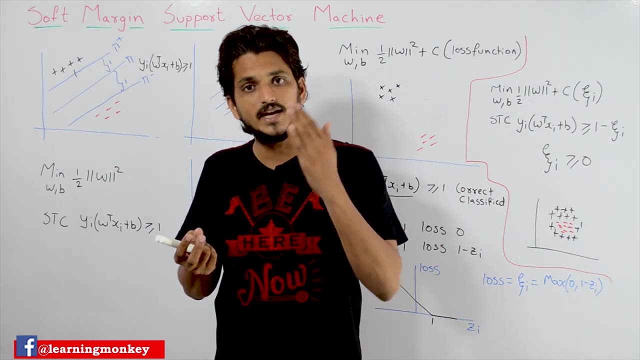 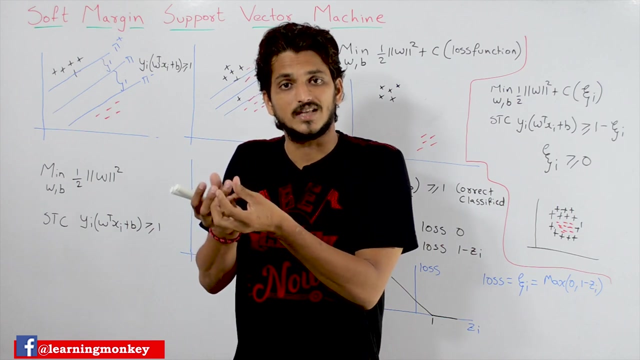 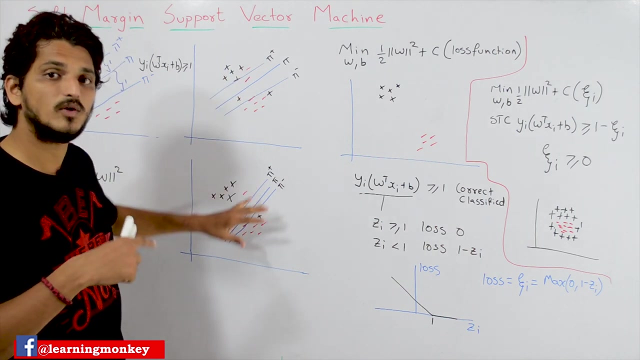 and we try to identify a line that minimizes the class. the same concept we applied in linear regression. also, we identified a loss function and we- I we try to identify a line that minimizes that loss. the same way, the same way, in order to say which one is the best one. what we have to do? we have to 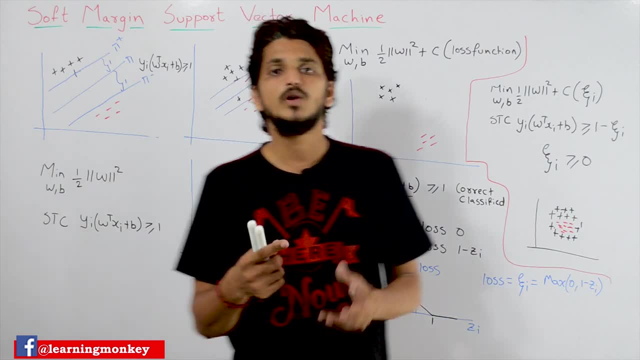 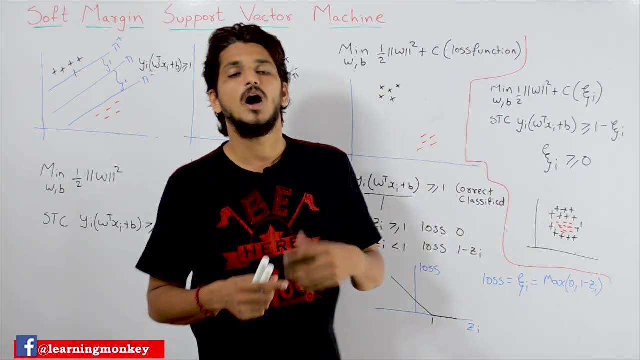 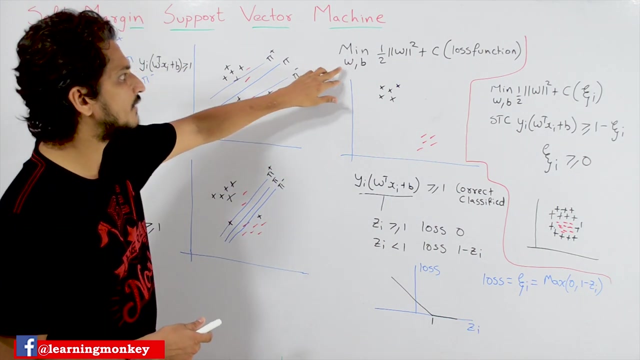 identify a loss function and we try to minimize that loss. so in this class we will understand about loss function. we define the loss function and optimization problem. so our optimization problem will be like this: minimum of w, comma B. for what W and B? we are having minimum of this function. what's the? 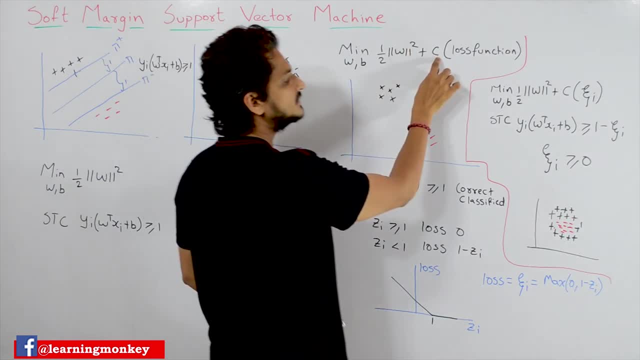 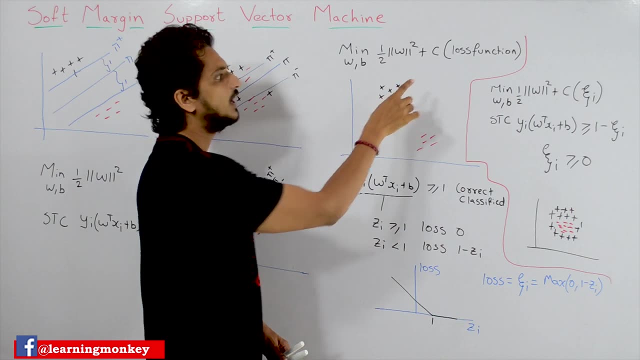 function is a 1 by 2 norm W square plus C into loss function, not a. define the last function. we have to define the last function. this is our optimization problem. forget about C in this class. we'll discuss what's the C, what's the use of C, in our next class. 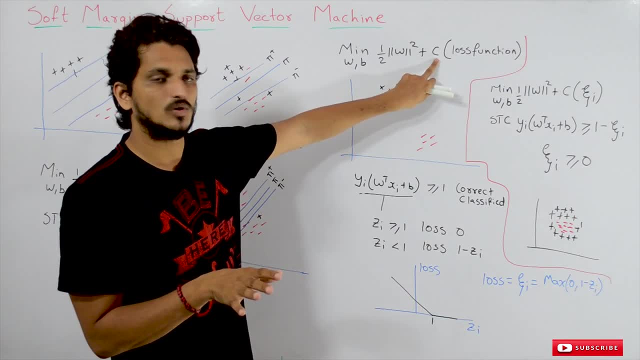 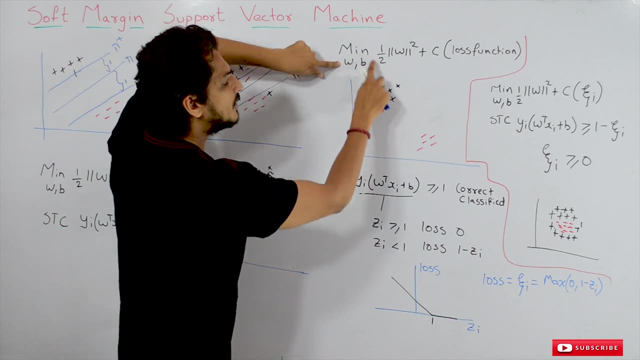 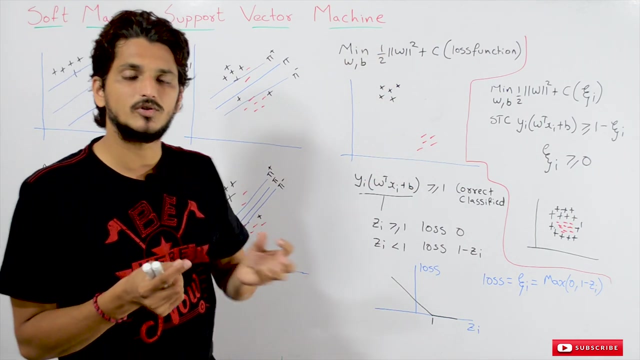 consider it as a constant. so what's this optimization problem is saying: identify a line for which line we are having minimum of this summation value. so what's the optimization value? 1 by 2, norm W square. we are trying to minimize with norm W square. at the same time, we are trying to minimize the loss function also, if you. 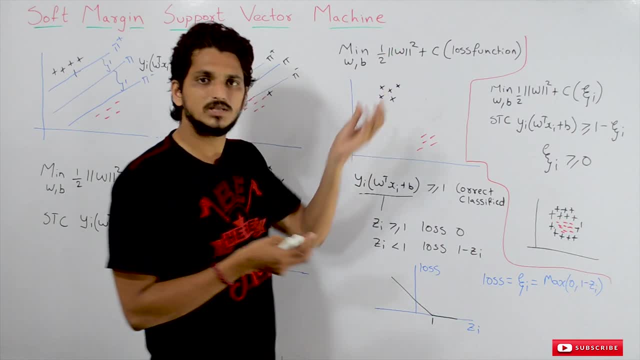 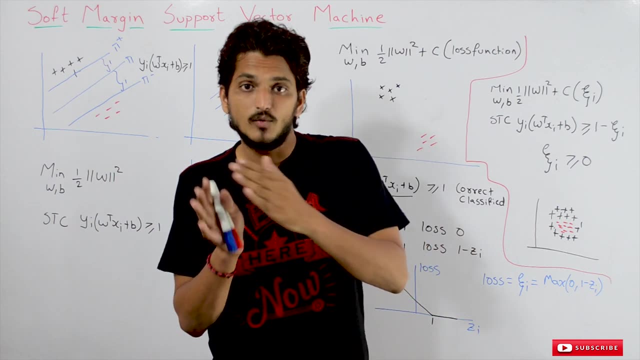 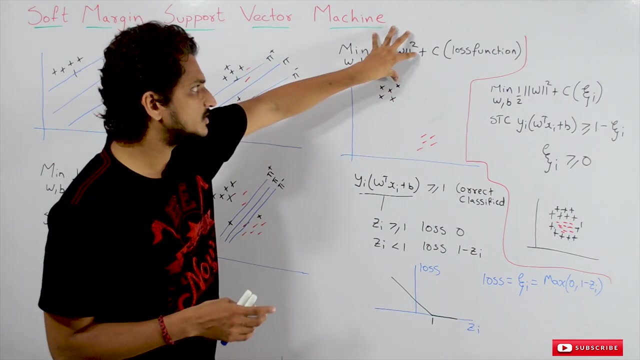 are trying to minimize this loss function. this norm, W square, means we are trying to maximize the margin. at the same time, we are taking the summation of we are trying to minimize the loss function also. so what's this optimization problem is doing is, if you solve this optimization problem, what's? 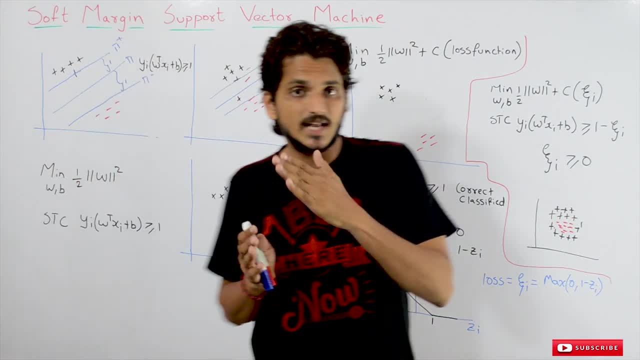 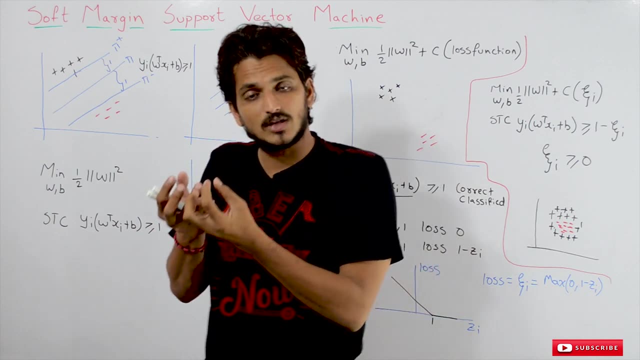 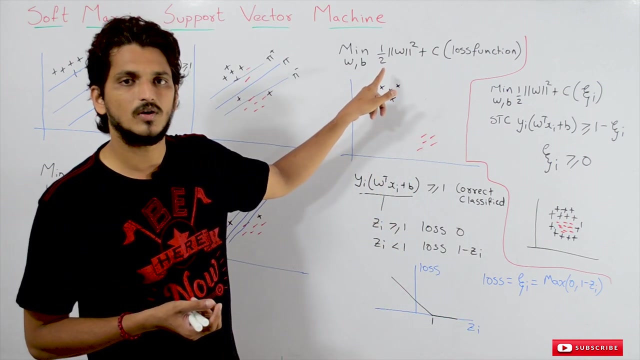 this optimization problem will identify is it will identify a line that maximizes the margin and, at the same time, minimizes the loss. that line will be identified for our soft margin svm. okay, in this optimization problem, we know about this- the same thing from hard margin svm when we 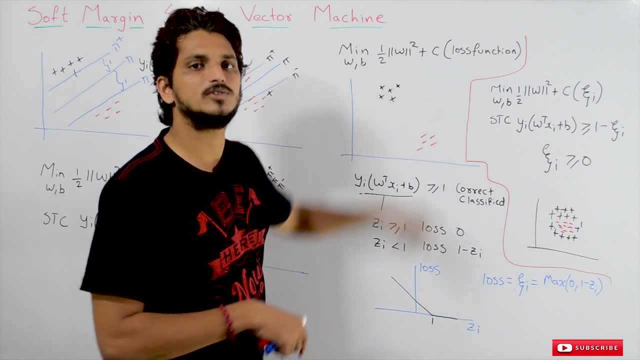 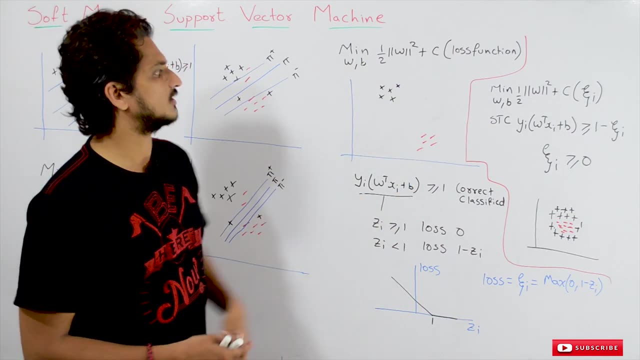 have to identify this loss function. we will discuss about this loss function in this class. so now let's take an example and understand what's this loss function, how we define the loss function for understanding purpose. we we are given so much of gap here we are taking a. 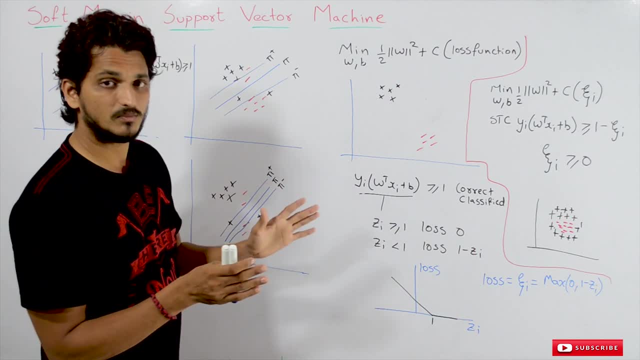 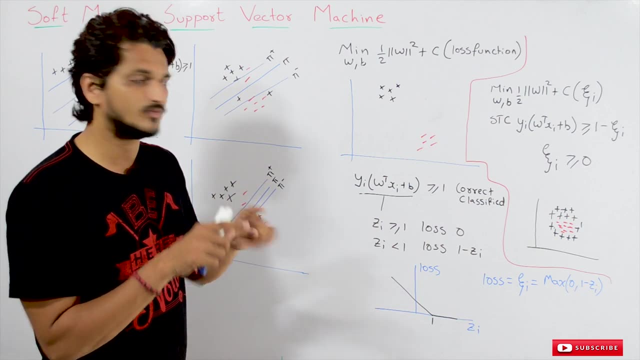 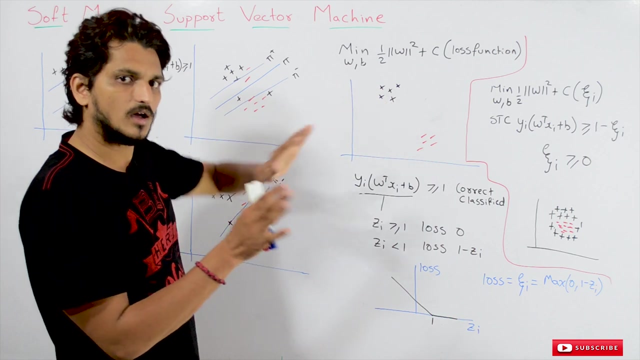 data set which is linearly separable, but our data set is not linearly separable. we have to add points now and we will discuss about the loss function. that's why, for now, these are our data points. we will add some data points here, okay, but for understanding purpose, we are giving so much. 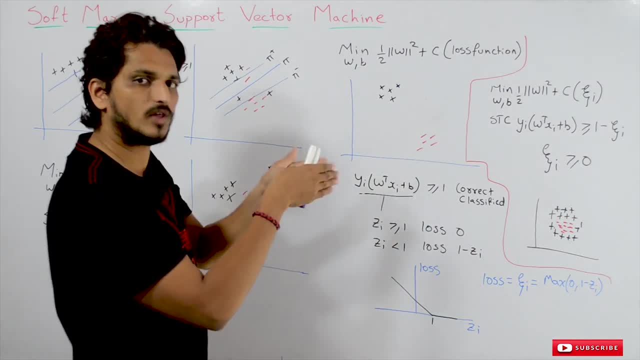 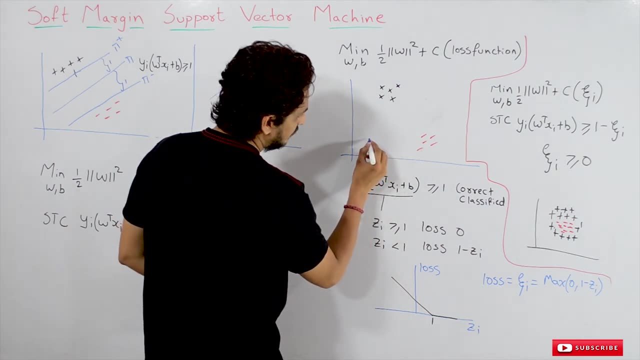 data points here. okay, but for understanding purpose we are giving so much data points here, okay, but for purpose. so much of gap is given. we have to write some down, write something here. that's why we have given some gap, okay. so suppose, if our support vector machine has identified this line as the 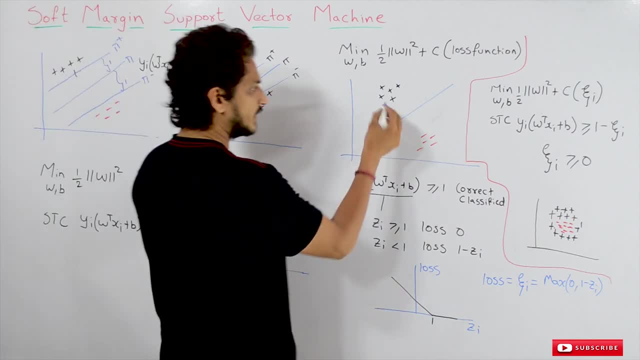 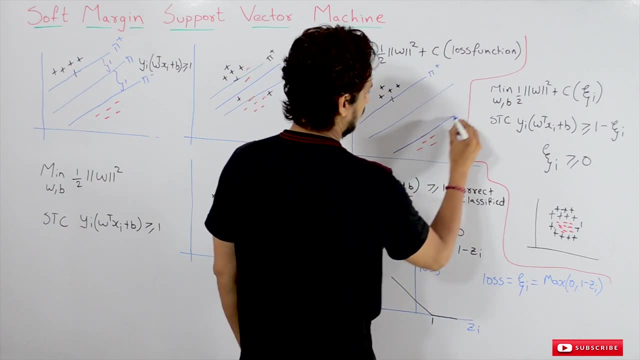 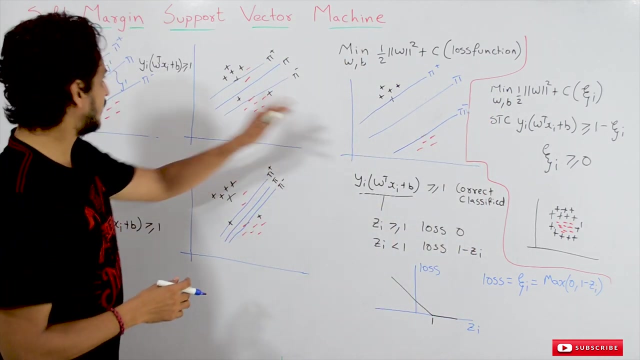 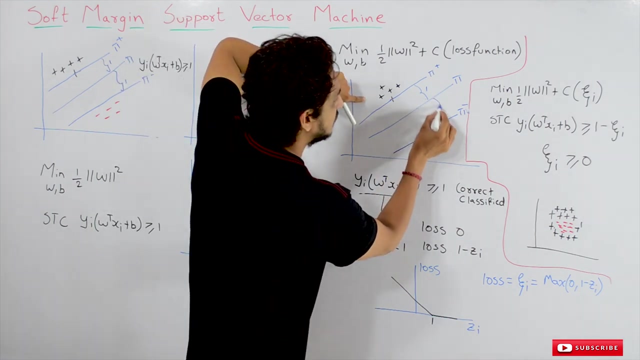 best line. so, when coming to, this is the best line. this line we call it as pi plus, this line we call it as pi minus, this we call it as pi. so what we have defined in hard margin, SVM, this functional margin will be 1. this functional margin will be 1. okay, the. if you substitute this point in the 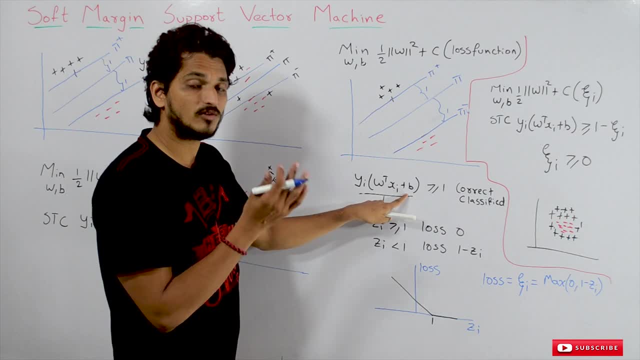 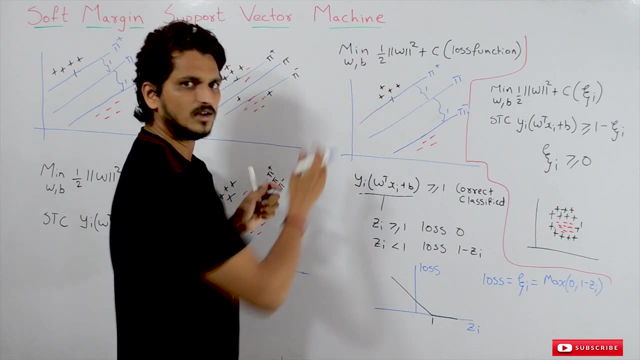 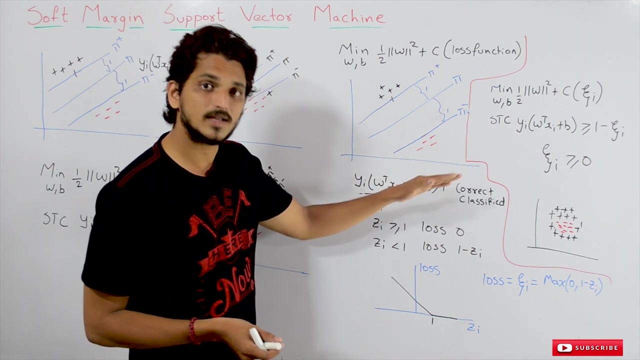 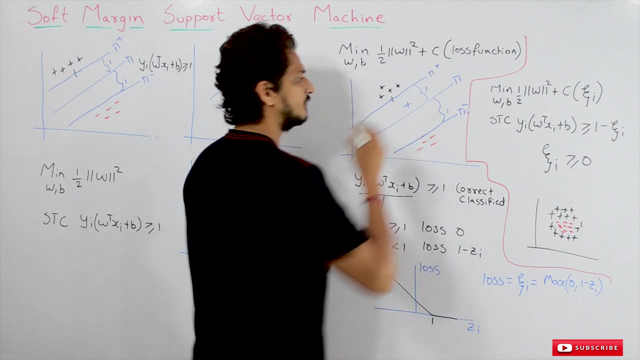 equation yi w: transpose xi plus b: if it is greater than or equal to 1 means the point is above this line. if the point is above this line, this line means correctly classified. the same way, if a negative point is below this line means correctly classified. what happens if the point is here? if a positive point is there here, above? 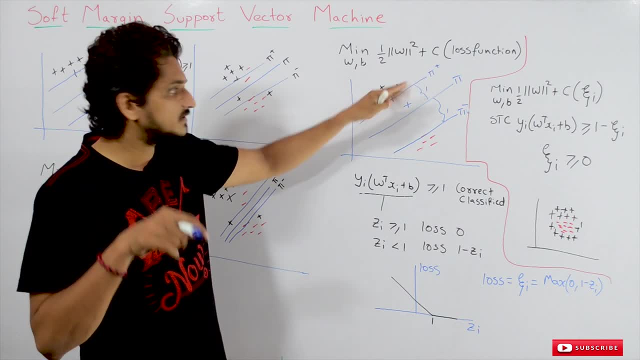 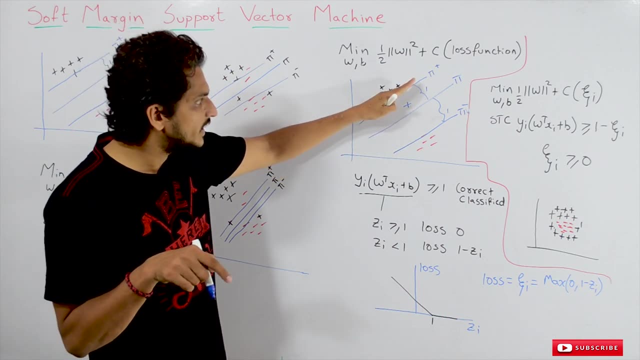 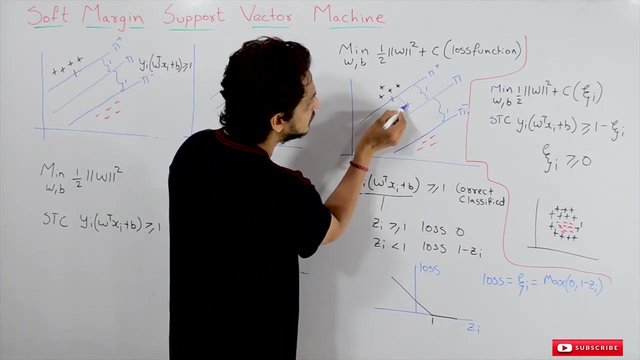 this line, we are considering it as correctly classified means it is not correctly classified means we have to assign some loss. how we assign so here onwards, from above this line, we are considering it as a correctly classified, so we calculate loss from here to here. this we call it. 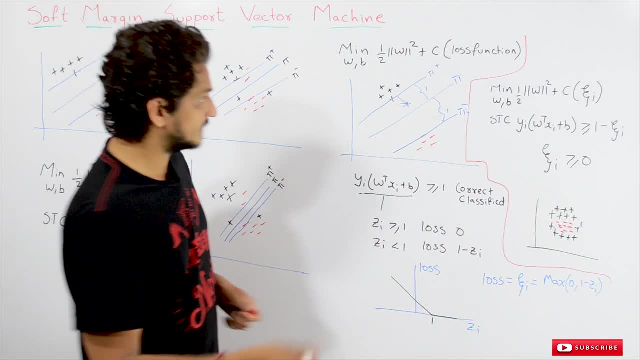 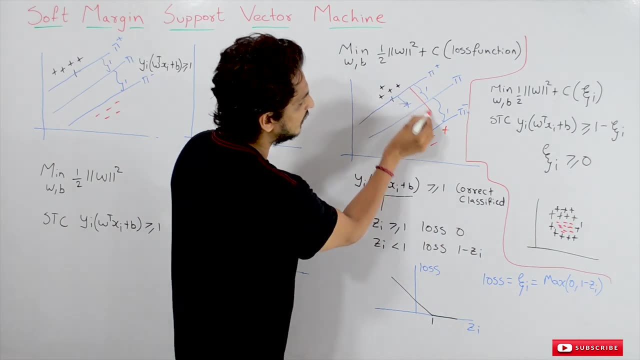 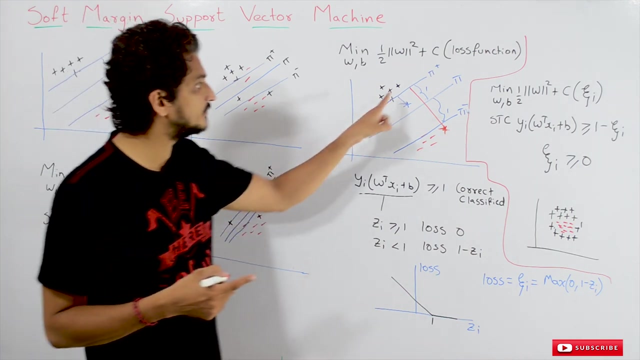 as loss. okay, the same way, if our pause, if a positive point is there here. how we calculate the loss, this value, we call it as loss. so clearly understand from where we are calculating the loss: from this line. do we really know this line? which line we will identify? we will identify. 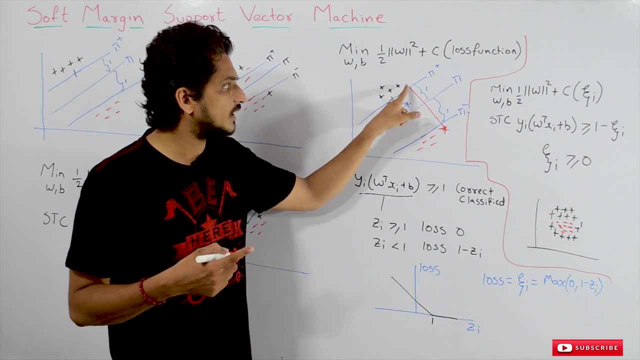 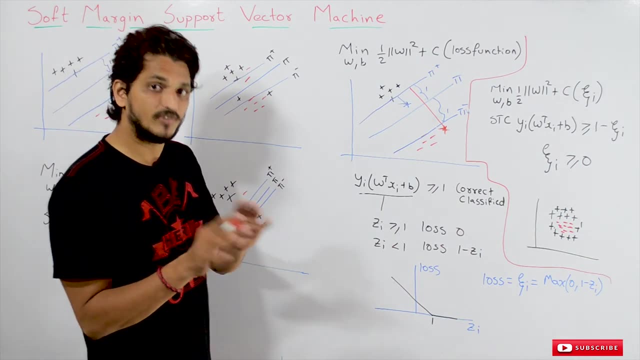 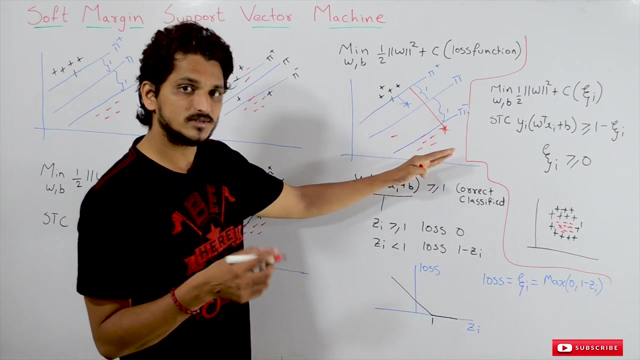 this line, but then how we calculate the value from here. that is what we'll understand in this class. we'll get the same way, if a negative point is present here, what we discussed. if the point is above this, below this line, we are considering it as correctly classified means we will assign a. 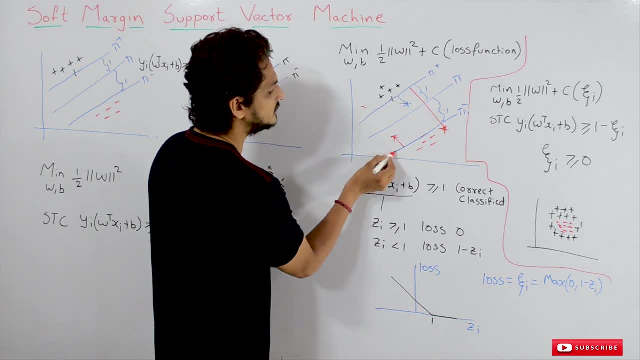 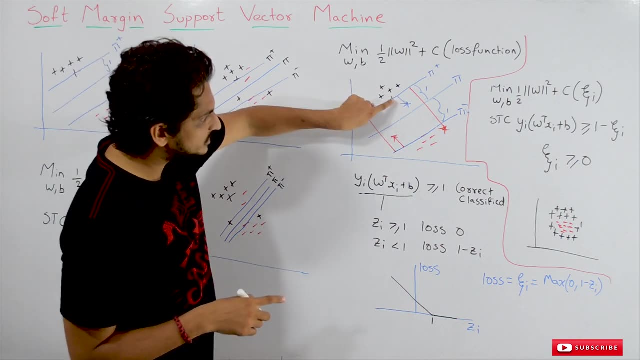 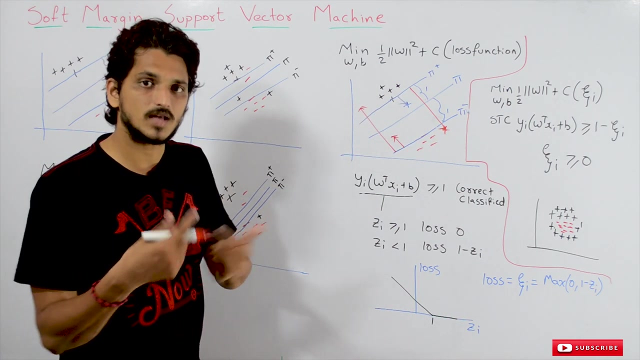 loss. and the same way, if the point is here, we will assign a loss. like this, what we understand from this diagram: if the positive point is near to this line, we have to assign less loss. if the positive point is away from this line, we have to give some large loss value. the same way if a negative point. 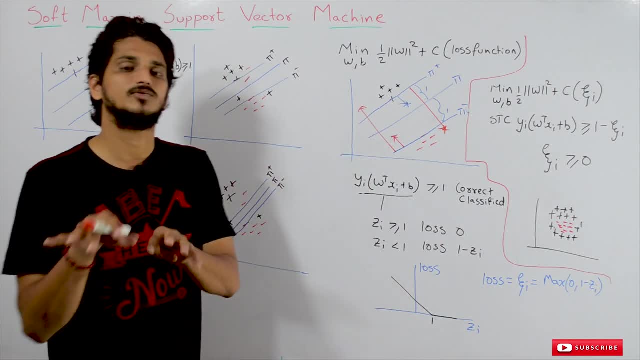 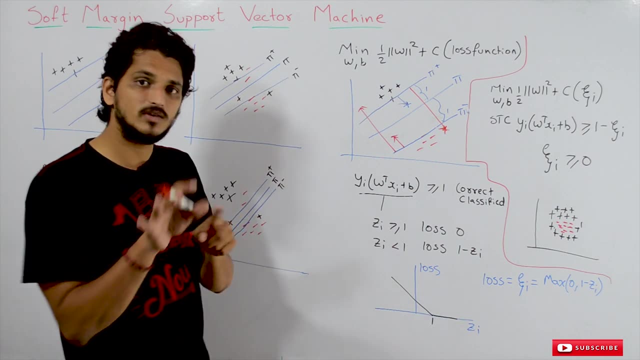 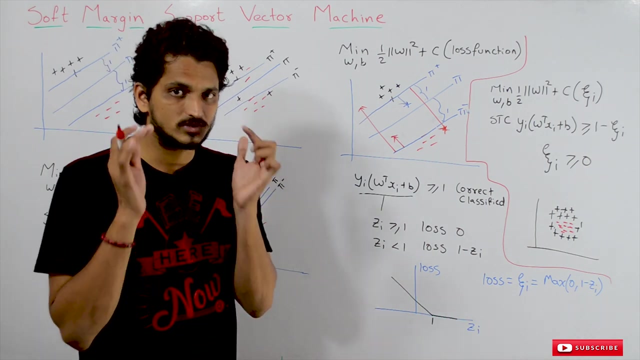 is away from this line, we have to give large loss value. if it is near to this line, we have to give an less loss value. so how we assign this loss? what's the equation? we will identify this equation. so what we do here is: you please concentrate, because it's a little bit confusing. 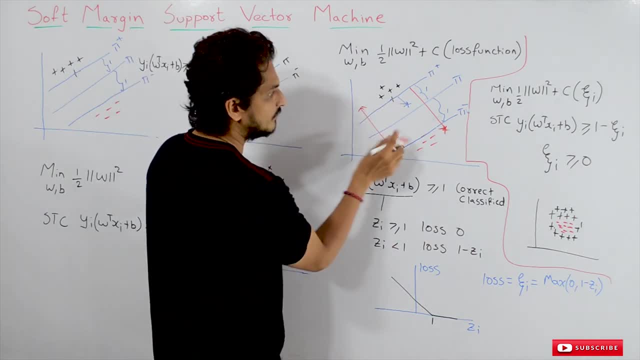 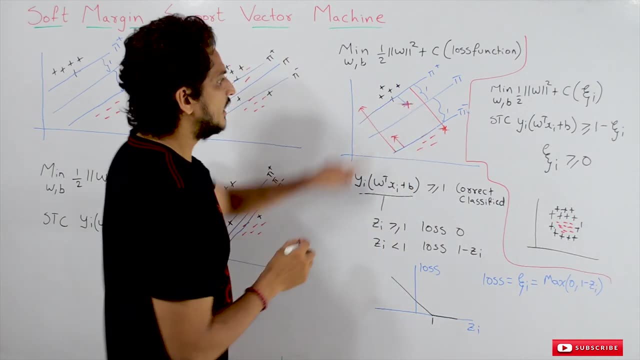 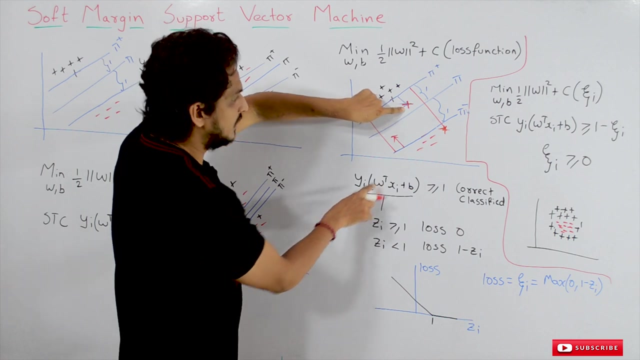 we have to identify loss like this, but we know this line equation. if you identify this line equation, suppose, take this point. if you substitute this point in this equation, what's the yi value? positive value means plus one. if you substitute this point in this equation, this equation is: 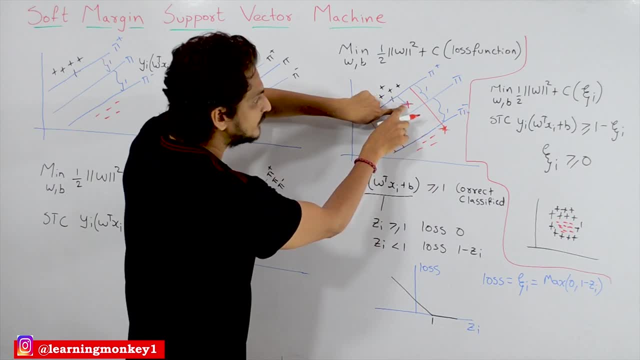 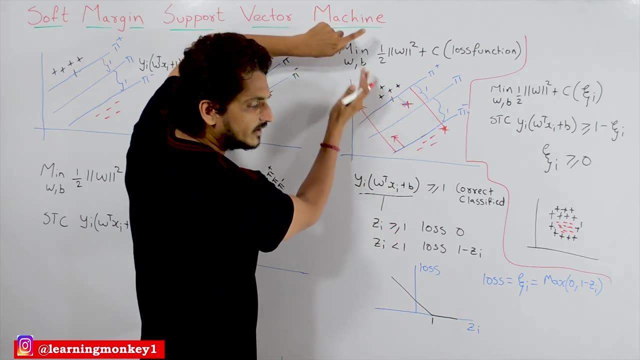 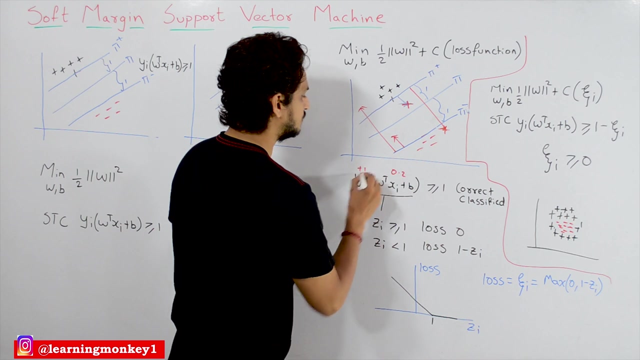 this line equation. okay, if you substitute it. what we are calculating here? functional margin. if the functional margin- because this point is on this side- the functional margin will be positive. assume the functional margin value is 0.2. this plus one plus one into 0.2, what's the value you? 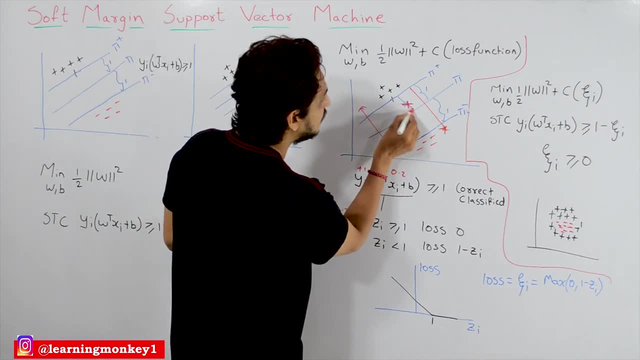 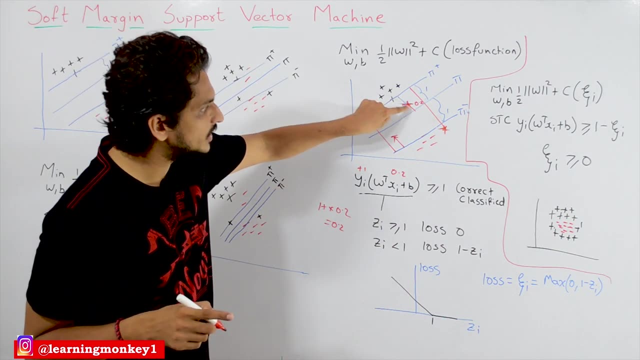 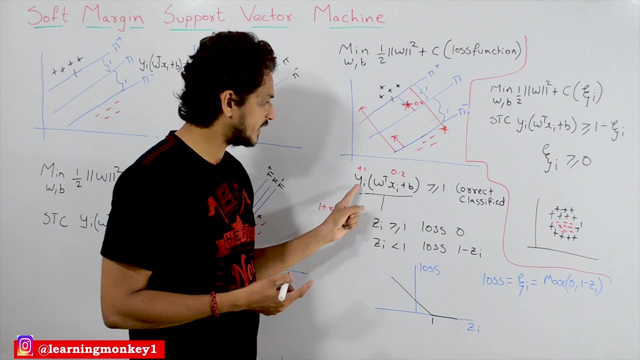 got 0.2. so what's that value? this value is 0.2 for loss. what we have to identify from here to here, we have to identify how we identify here- is: we consider this equation as zi, yi, w. transpose xi plus b is called as zi. if zi is greater than or equal to one, we call it as: 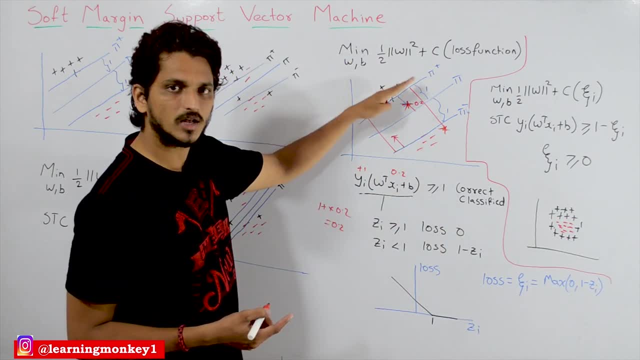 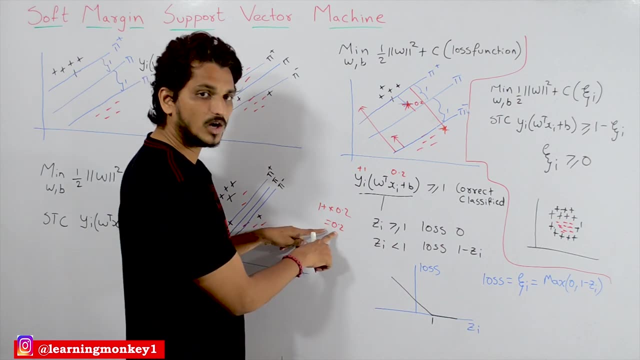 loss is equal to zero means the point is above this line. if zi is less than one, loss is equal to 1 minus zi. 1 minus zi. see what's the zi value. we got here: 0.2. 1 minus zi means 1 minus 0.2. 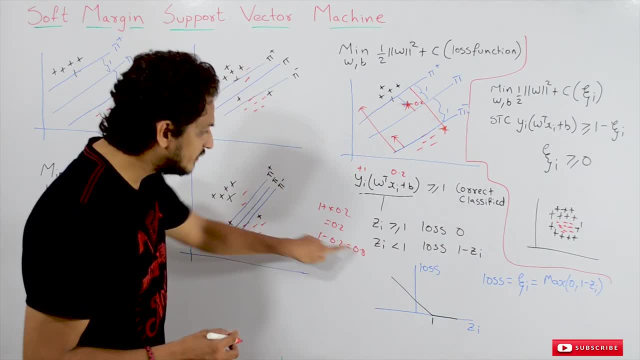 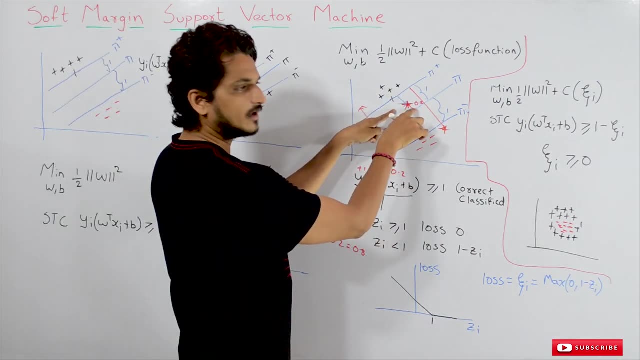 that is equal to 0.8, so why we did 1 minus 0.2. we know that this functional margin is 1. what's the functional margin value? we got here, 0.2. 1 minus 0.2, which one will get from that side. 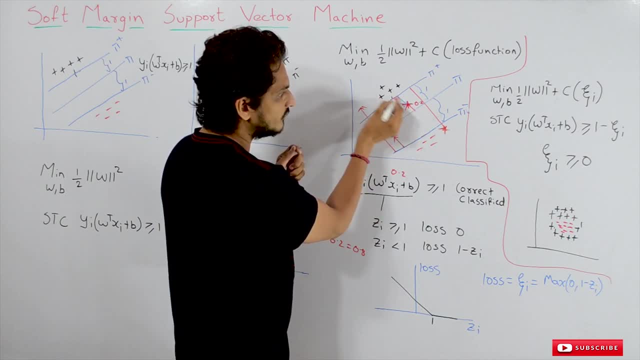 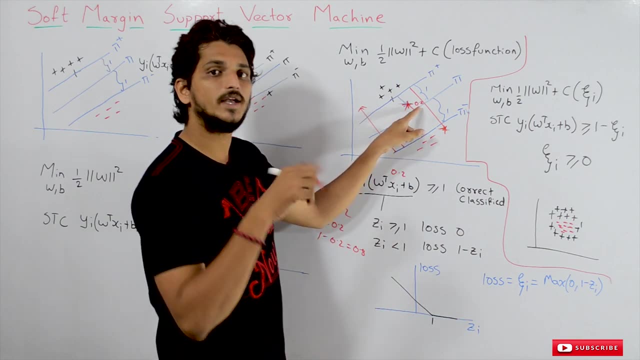 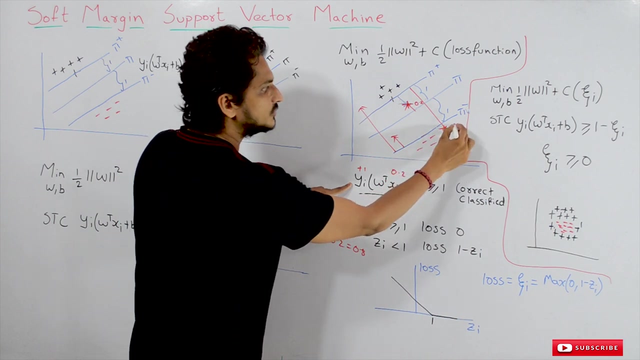 this is the value we will get, because this total functional margin is a 1.. so 0.2, 1 minus 0.2, 0.8. the same way, if the point is here, if you substitute this point in this equation, actual value is positive. this is positive. point yi means a plus. 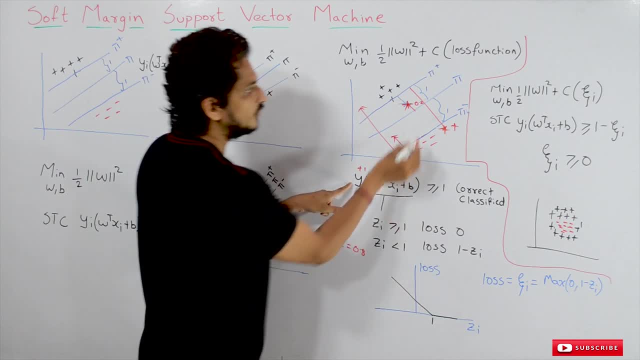 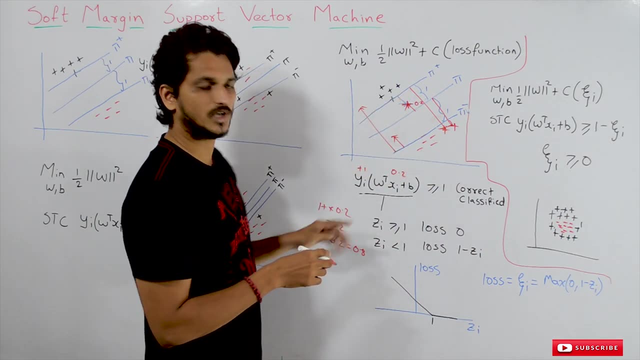 1. if you substitute in this equation the functional margin value, will get the functional margin value. from here we will get negative value. why? because this is on the opposite side of this line means we will get negative value, so positive into negative value. first, suppose we got as minus 5. 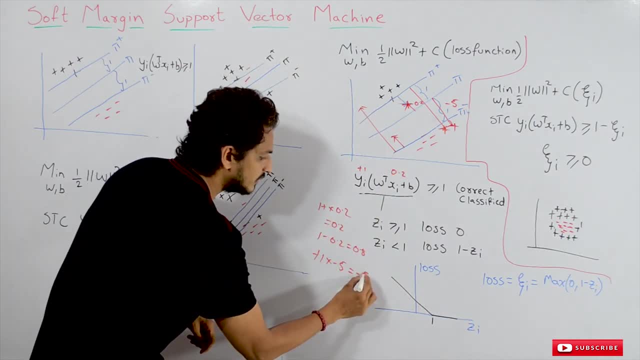 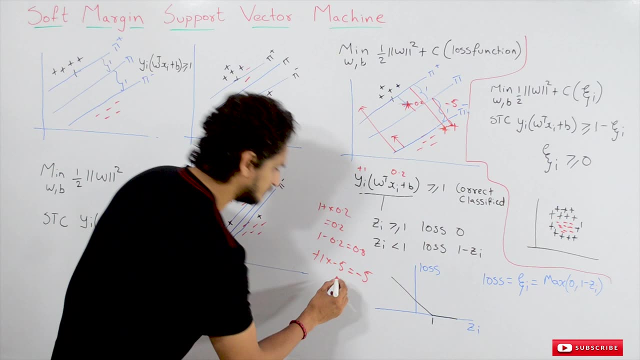 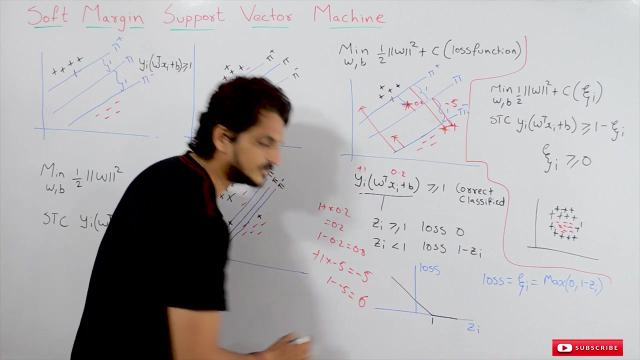 plus 1 into minus 5. we got, we will get it as minus 5. but what we are doing for the loss function loss is equal to 1 minus minus 5. 1 minus zi is minus 5 minus 5. that is equal to 1 plus 5. that is equal to 6. that's the loss. the same way we will identify loss to negative. 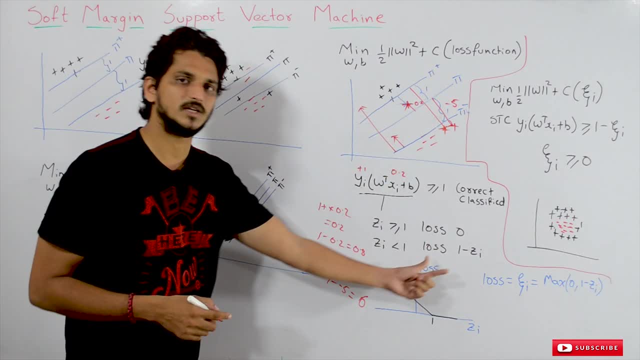 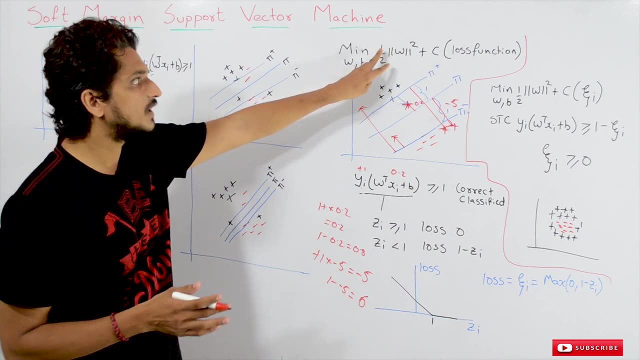 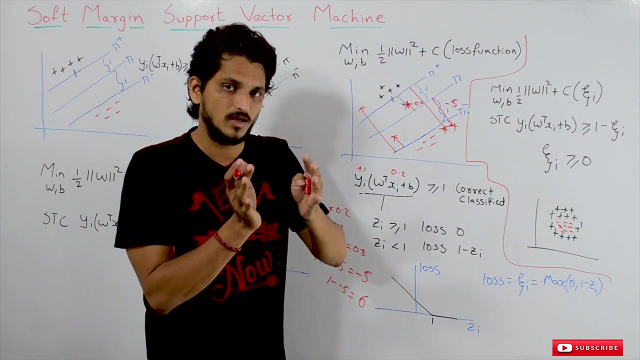 points from this side the same equation: 1 minus zi. this is how we calculate the loss. so what's our optimization problem? our optimization problem has to reduce the loss. at the same time, it has to increase the margin for which line we are getting this value minimum. 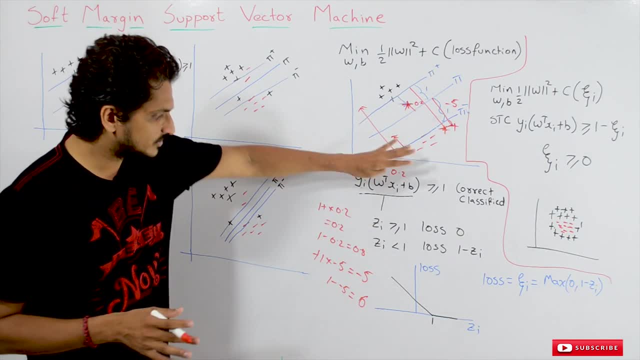 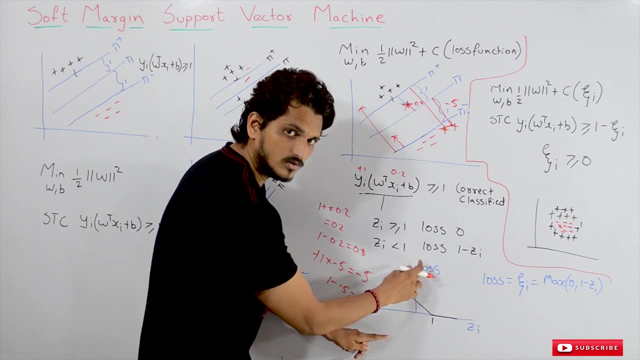 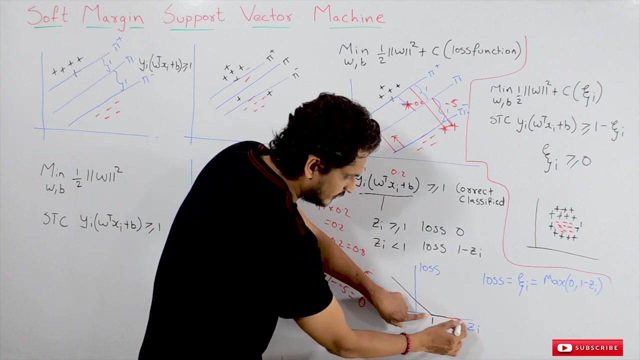 value, that line will be identified. so let's take it as a graph. if you take x on the x axis, we are taking zi value. on the y axis, we are taking loss value. so if our zi value is greater than or equal to one, what's the loss? zero loss is zero and the same time, if it is less than one, our loss. 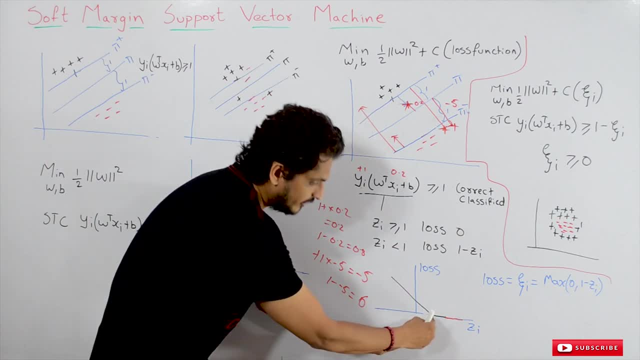 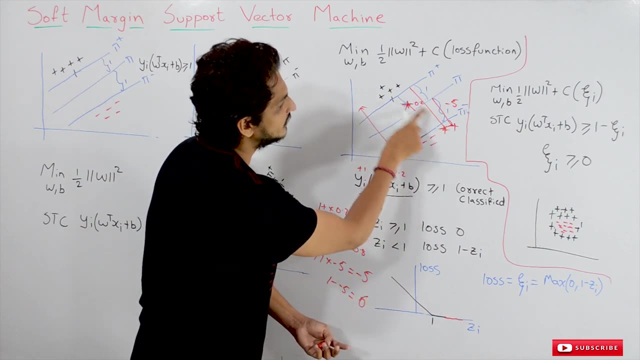 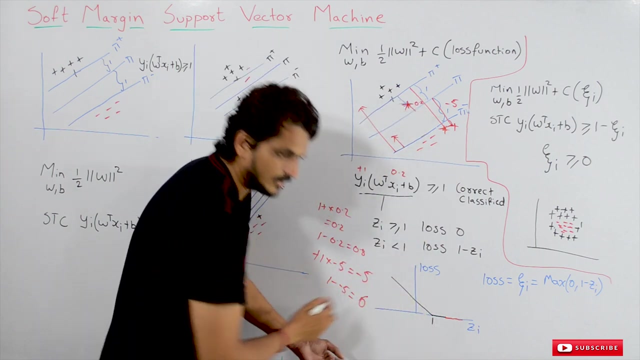 value has to be increased. why it is increasing. if, if the loss value is moving towards negative side, loss will be increasing. that's what we understand here. if it is minus, minus 5, minus, the loss value increases. that's why this line is increasing. so this function, we call it as hinge loss. this 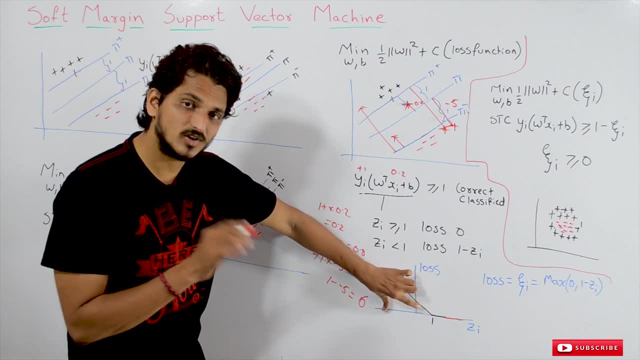 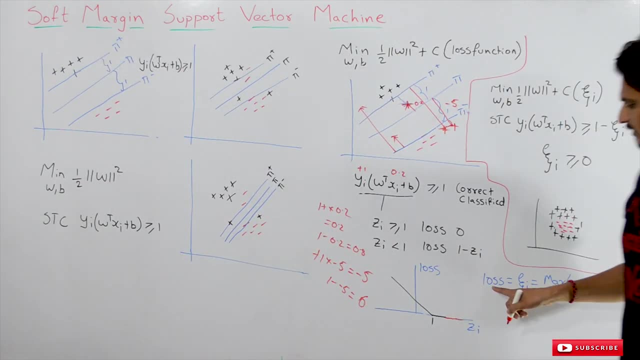 function. we call it as hinge loss. this function actually maps to our actual problem: how we convert the loss. that hinge loss is equal to. the loss is equal to zeta i is equal to- we call it a slack variable: zeta i. zeta i is equal to maximum of 0 comma 1 minus z, maximum of 0 comma 1 minus zi. 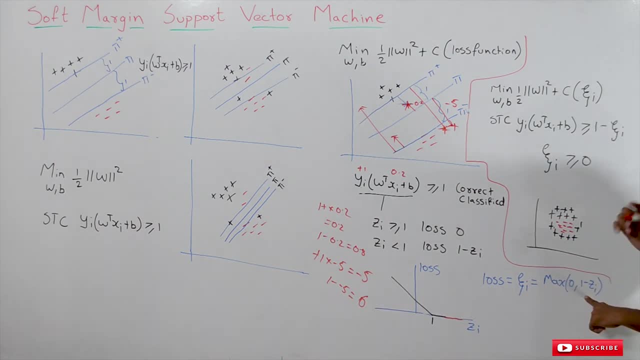 so why? why? maximum of 0 comma 1 minus z day? you have to understand this. so zi greater than or equal to 1 means what's the loss? 0. so maximum of 0 comma 1 minus zi z greater than or equal to 0. 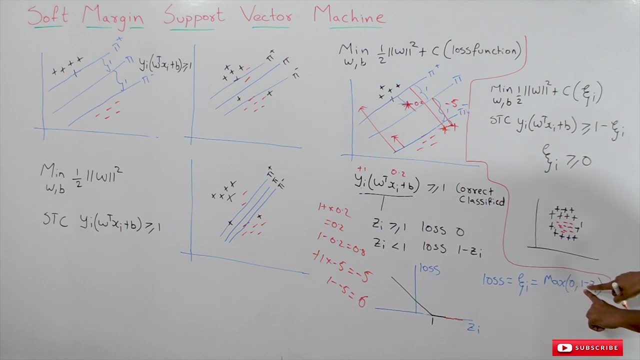 greater than or equal to 1 means maximum of 0 comma 1 minus. if z greater than or equal to 1, 1 minus zi will be negative value. so maximum of 0 comma. negative value means 0. so 0 is bigger than negative value. which one will be picked? maximum of 0 will be considered. that's why loss is equal to. 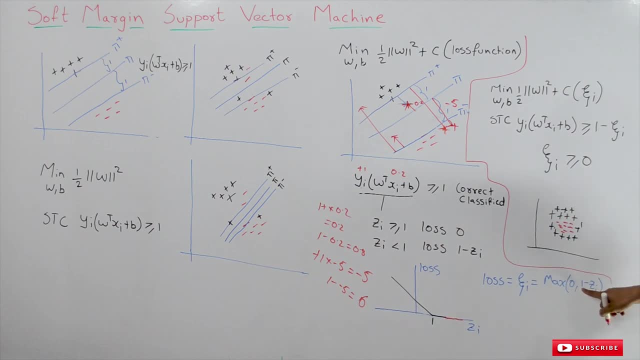 0.. the same way, if zi is less than 1, what's the value of 1 minus zi? it is positive value. so maximum of 0 comma 1 minus zi is equal to 0.. 0 comma positive value, which one will be considered positive value will. 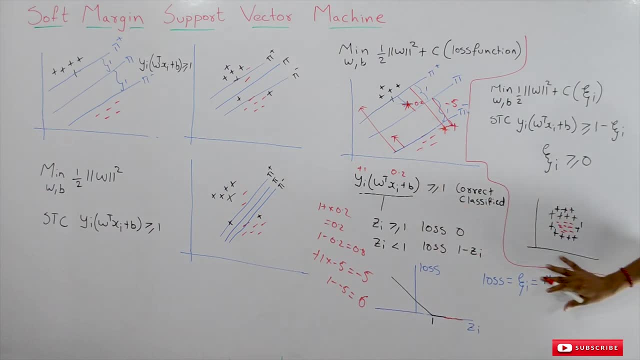 be considered. so this problem is converted into this equation: maximum of 0 comma 1 minus zeta. if zeta is greater than or equal to 1, consider the maximum of 0 comma. 1 minus zi will be negative value, so we'll consider 0, otherwise 1 minus zeta. this is our loss function. we call it as: 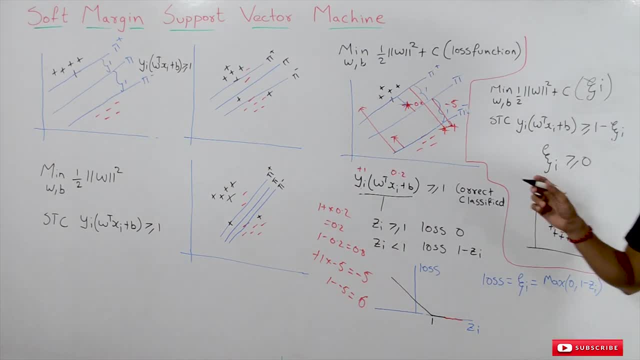 hinz loss. hence our optimization problem will be minimum of w comma b. sorry i have written wrong here. zeta is the loss value, but we have to calculate loss for all the data points means it will be: sigma i is equal to 1 to m zeta i value. 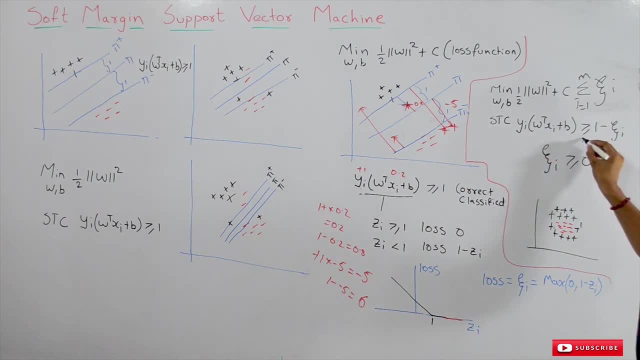 for all the points the same way. our constraint should be satisfied for f, for i is equal to 1 to m. this is the optimization problem. what's our optimization problem is minimum w minus zi, half norm w square plus c into sigma i is equal to 1 to m. zeta i, zeta i is the loss value subjected. 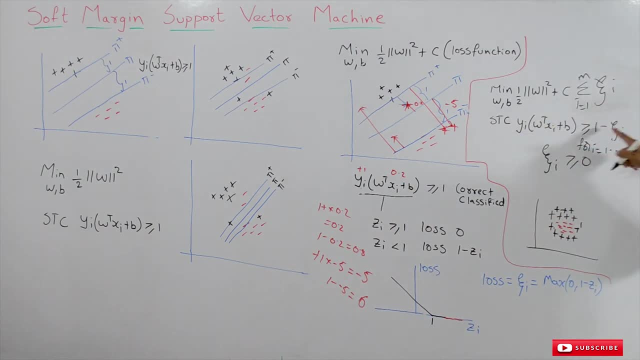 to constraints. y, i, w. transpose x: i plus b. greater than or equal to 1, minus zeta i. for all the one i is equal to 1 to m points and zeta i should be greater than or equal to 0. see here zeta i will. 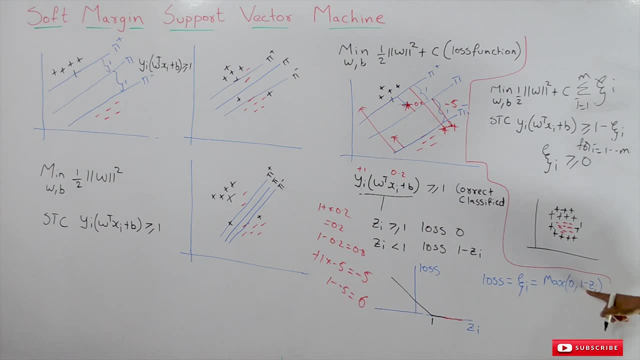 not be negative either. it will be 0. if it is negative, it is taking the maximum of 0 comma negative value, so 0 will be there. it won't be negative value. zeta i value will not be negative value, so it will be 0 or greater than 0. so that's why we had the constraint zeta i greater than or. 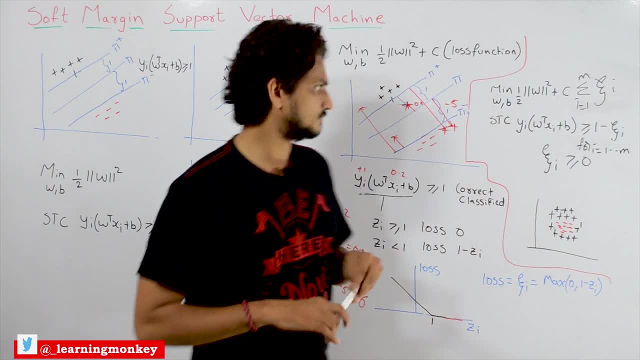 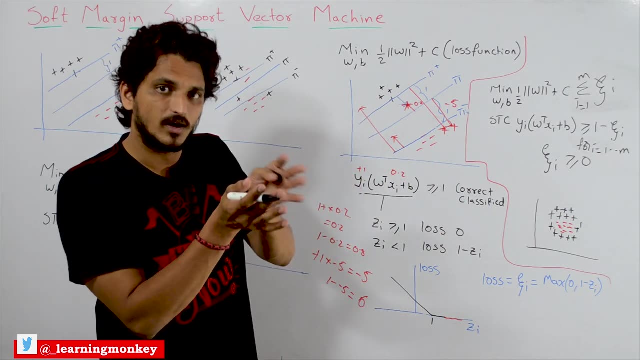 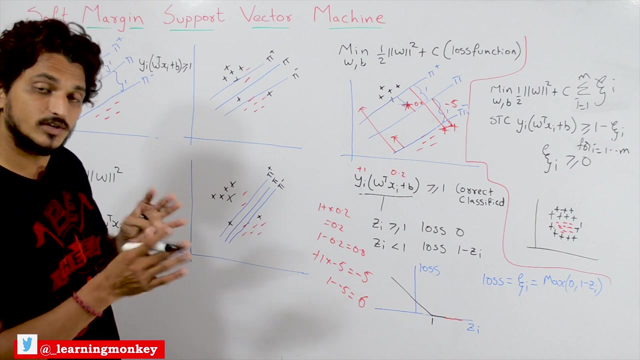 equal to 0. so what's this optimization problem is doing? it will identify a line that gives the maximum of the margin and minimum of the loss function in these two lines. it will identify a line that gives the maximum of the margin and minimum of the loss function in these two lines. 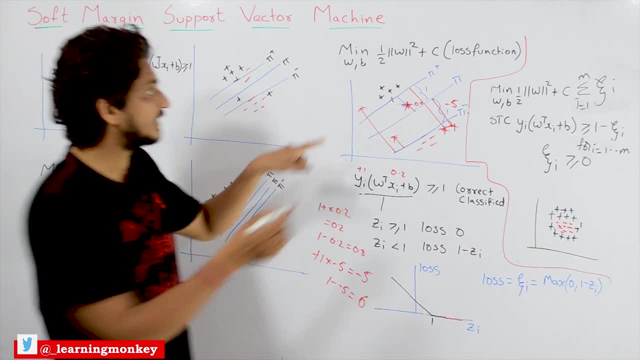 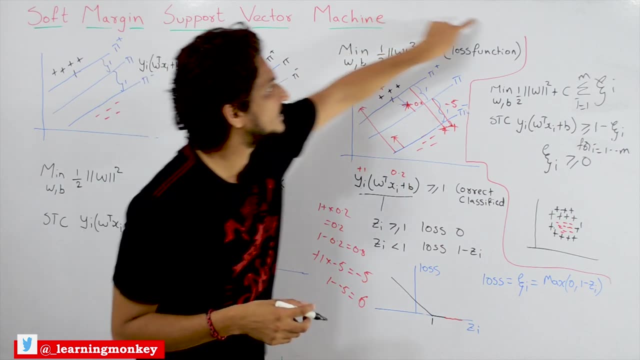 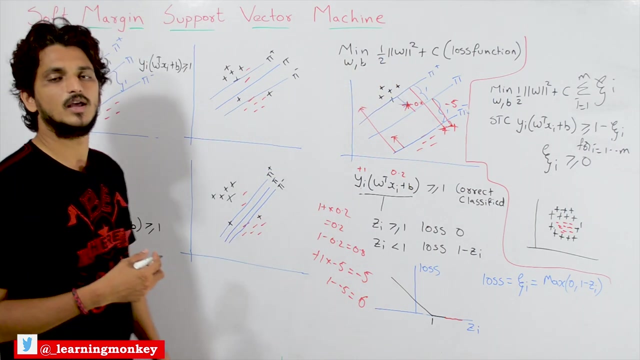 use the maximum margin and minimum loss. so it will consider both these values, for which w and b values. we are having this entire function: minimum that will be considered. that value will be considered, that w, b will be considered. this is what our optimization problem is: how to solve this. 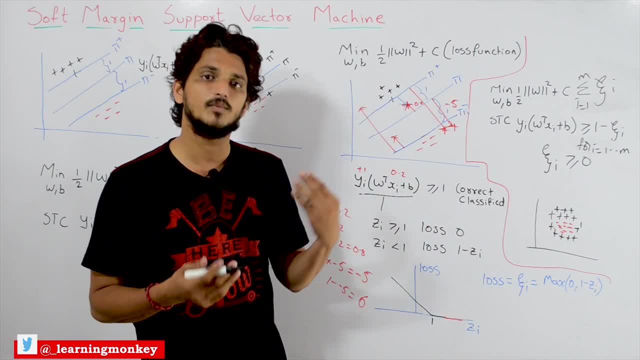 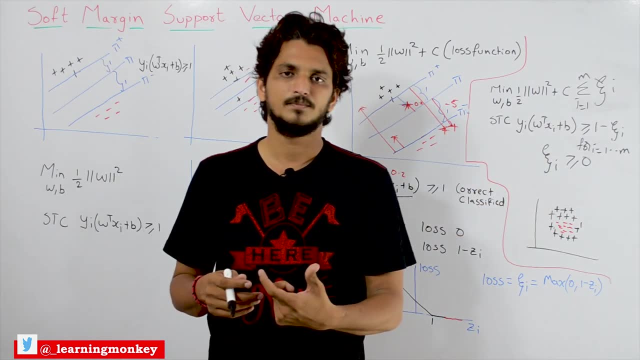 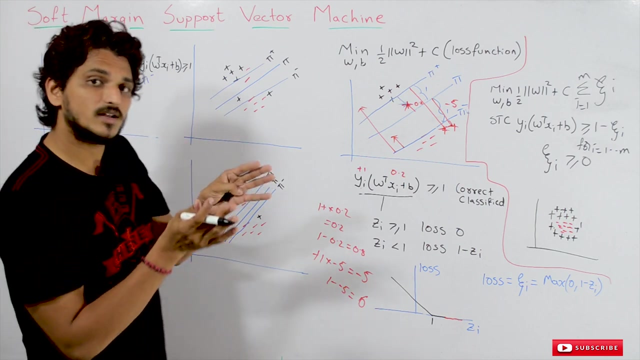 optimization problem. the same way, in our hard margin svm, how we solve the optimization problem, we convert this optimization problem into dual problem and we'll solve the dual problem. and coming to one more important point, see, when we consider this data set, this is almost linearly separable data. so what happens if it is not linearly separable data? let's take